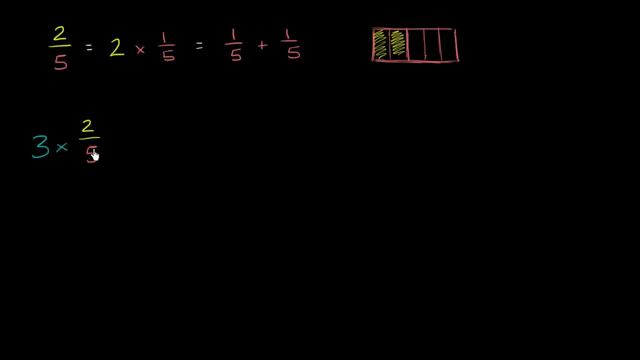 and based on what we just did here, think about what you think. What do you think this would be equivalent to? Well, we just saw that 2 fifths would be the same thing as: so let me just rewrite this as, instead of 3 times 2 fifths. 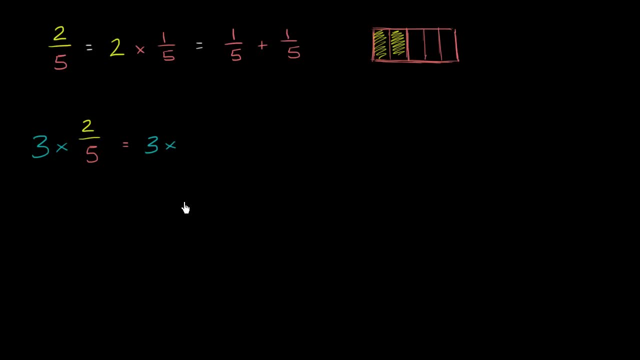 written like this: let me write 2 fifths like that. So this is the same thing as 3 times 2 times 1. fifth, 3 times 2 times 1. fifth times 1. fifth, And multiplication. we could multiply the 2 times the 1. 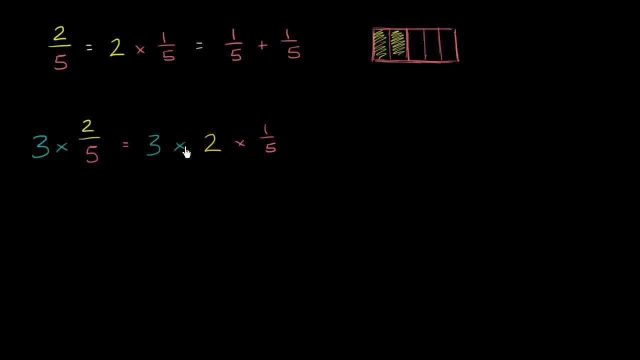 fifth first and then multiply. Or we could multiply the 3 times the 2 first and then multiply by the 1 fifth, So you could view this literally as being equal to 3 times 2 is, of course, 6.. 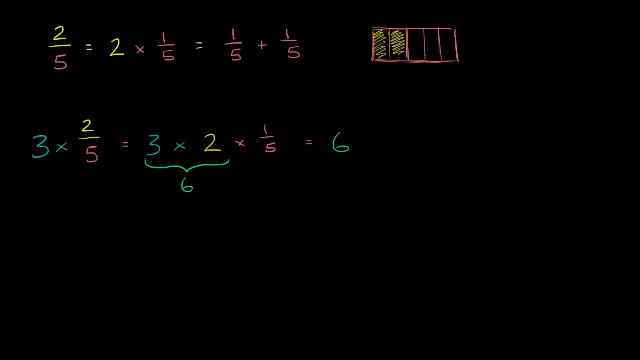 So this is the same thing as 6 times 1. fifth, And if we were to try to visualize that again, so that's a whole, that's another whole. Each of those wholes have been divided into 5 equal sections, And so we're going to color in 6 of them. 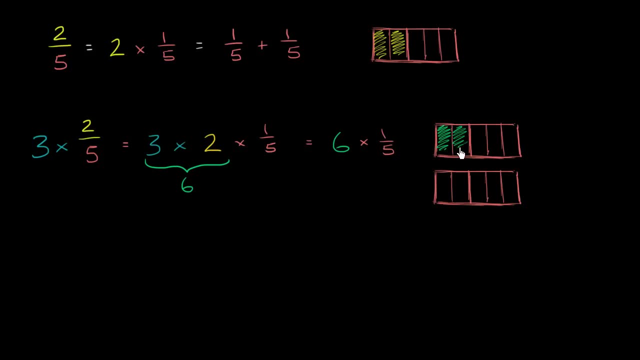 So that's the first fifth, second, fifth, third, fifth, fourth, fifth, fifth, fifth, and that gets us to a whole, And then we have 6 fifths just like that, So literally 3 times 2 fifths can be viewed as 6 fifths. 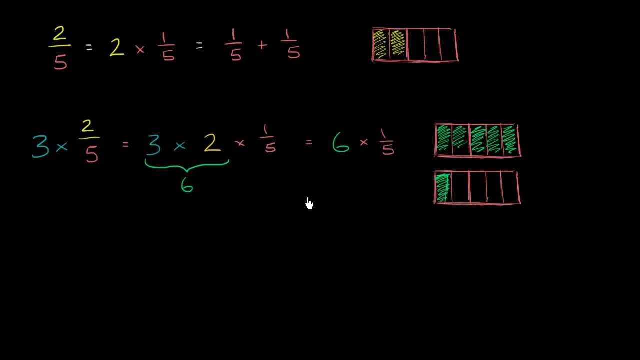 And, of course, 6 times 1 fifth or 6 fifths can be written as so this is equal to literally 6.5.. 6, let me do the same color- 6 fifths. 6 over 6 over 5.. 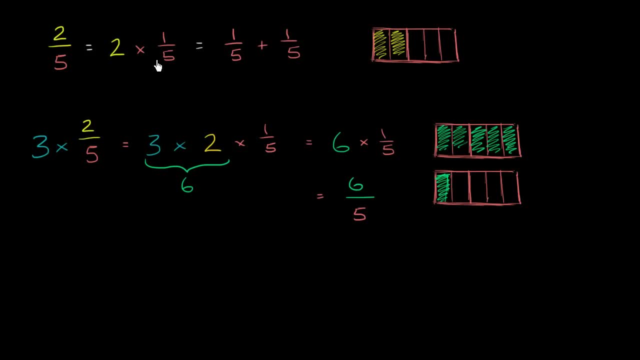 Now you might have said: well, what if we, instead of viewing 2 fifths as this, as we just did in this example, we view 2 fifths as 1 fifth plus 1 fifth? What would happen then? Well, let's try it out. 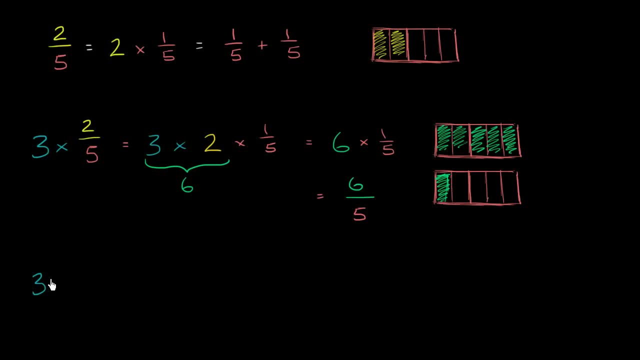 So 3 times 2 fifths. I'll rewrite it: 3 times 2 fifths, 2 over 5, 2 fifths Is the same. It's the same thing as 3 times 1 fifth plus 1 fifth. 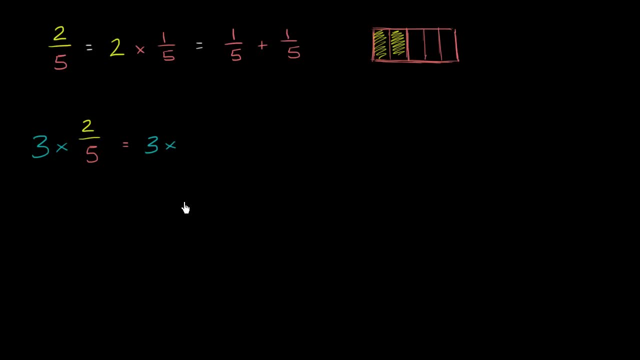 written like this: let me write 2 fifths like that. So this is the same thing as 3 times 2 times 1. fifth, 3 times 2 times 1. fifth times 1. fifth, And multiplication. we could multiply the 2 times the 1. 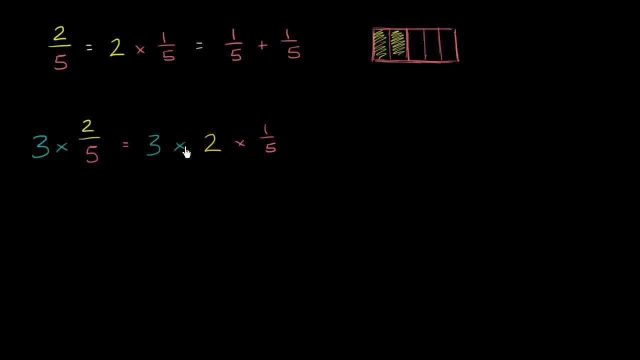 fifth first and then multiply. Or we could multiply the 3 times the 2 first and then multiply by the 1 fifth, So you could view this literally as being equal to 3 times 2 is, of course, 6.. 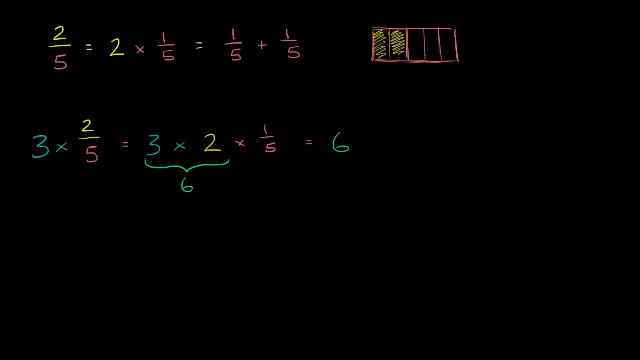 So this is the same thing as 6 times 1. fifth, And if we were to try to visualize that again, so that's a whole, that's another whole. Each of those wholes have been divided into 5 equal sections, And so we're going to color in 6 of them. 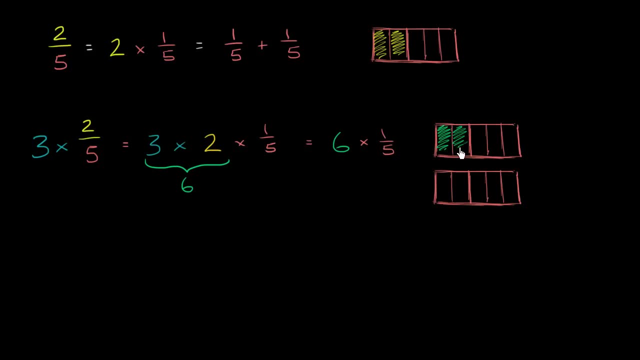 So that's the first fifth, second, fifth, third, fifth, fourth, fifth, fifth, fifth, and that gets us to a whole, And then we have 6 fifths just like that, So literally 3 times 2 fifths can be viewed as 6 fifths. 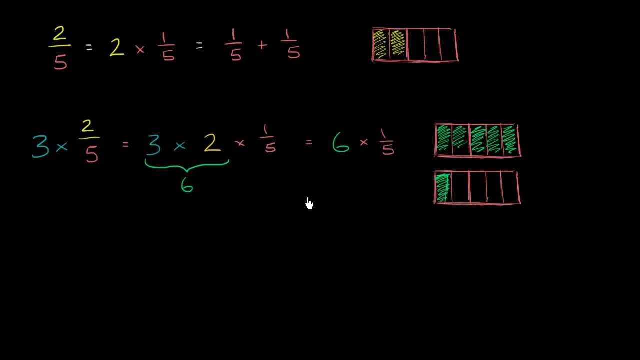 And, of course, 6 times 1 fifth or 6 fifths can be written as so this is equal to literally 6.5.. 6, let me do the same color- 6 fifths. 6 over 6 over 5.. 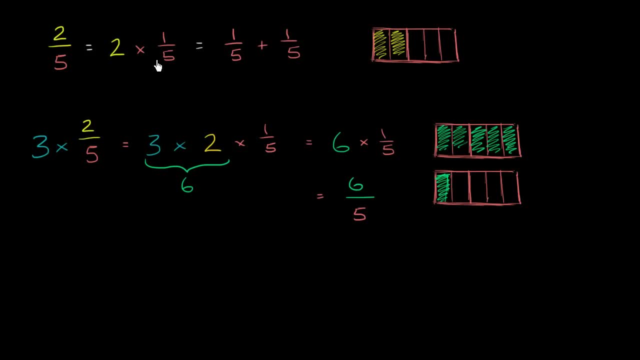 Now you might have said: well, what if we, instead of viewing 2 fifths as this, as we just did in this example, we view 2 fifths as 1 fifth plus 1 fifth? What would happen then? Well, let's try it out. 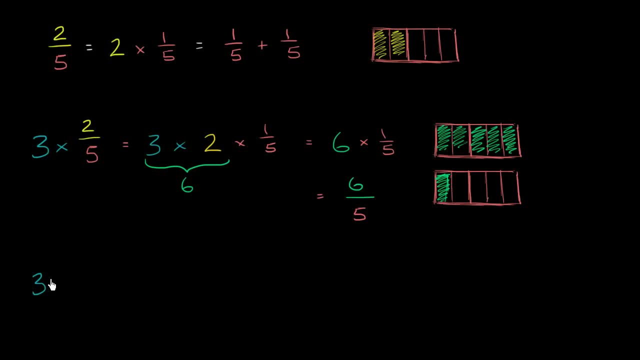 So 3 times 2 fifths. I'll rewrite it: 3 times 2 fifths, 2 over 5, 2 fifths Is the same. It's the same thing as 3 times 1 fifth plus 1 fifth. 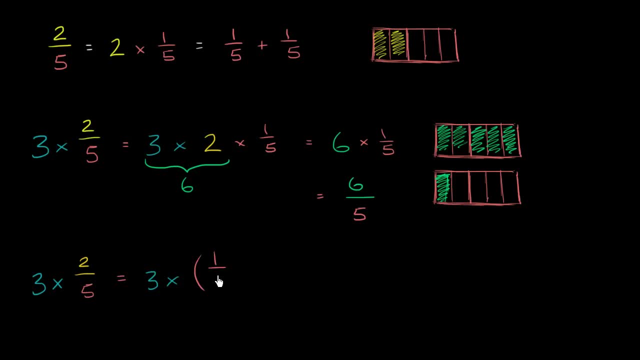 2 fifths is the same thing as 1 fifth plus 1 fifth, So 3 times 1 fifth plus 1 fifth, which would be equal to Well, I just have to have literally 3 of these added together. So it's going to be 1 fifth plus 1 fifth plus 1 fifth plus 1.